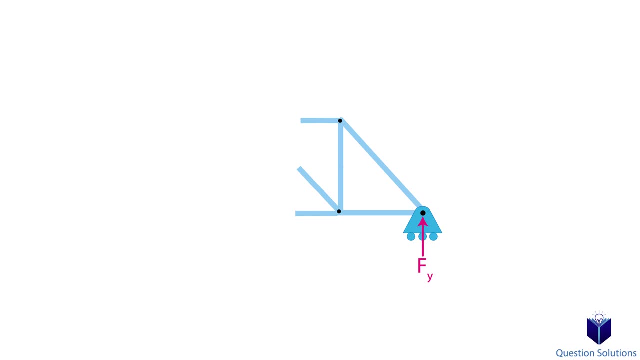 Now here's where things change. From this point on, the easiest way to think about this problem is to think of all of this as the truss and these cut members as external forces. In other words, this is one single object and these are the forces that are applied to it. 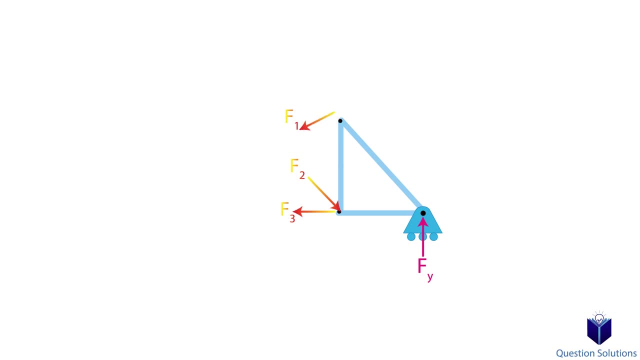 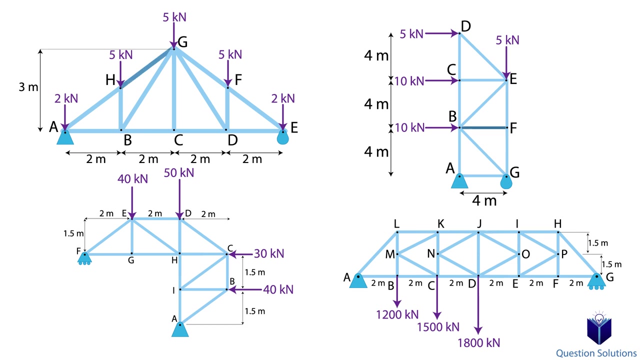 You can assume the direction of these forces. If you get a negative value, then it's opposite to your assumption. After that you can solve for these forces using equations of equilibrium or moment equations. This might be a bit confusing right now, but after we go through a few examples, hopefully you will have a firm. 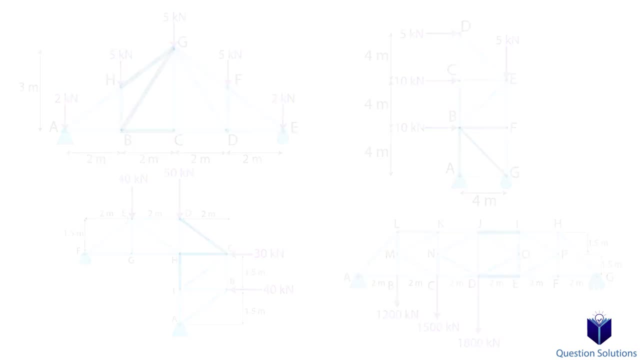 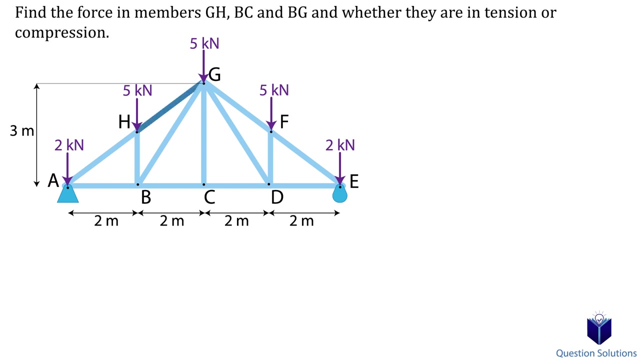 understanding of how to do this. Just a reminder from the previous video that if a force comes towards the pin, then that member is in compression and if a force leaves the pin, it's in tension. Let's take a look at this problem where we need to find the forces in members GH, BC and BG. 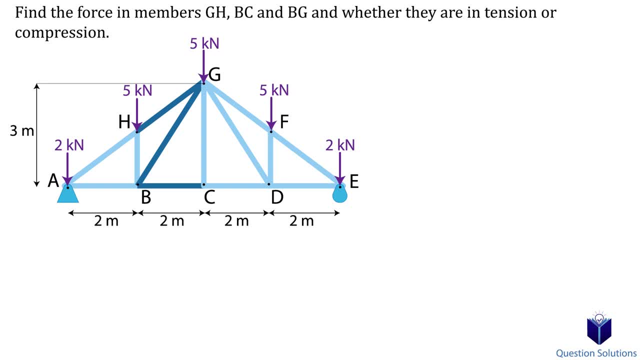 Since all of the unknowns we need to find are on the left side. we need to figure out the reactions of the forces. We can write a moment equation about point E which allows us to directly solve for the vertical reaction. We can see that there won't be an x-reaction at pin A, since there are 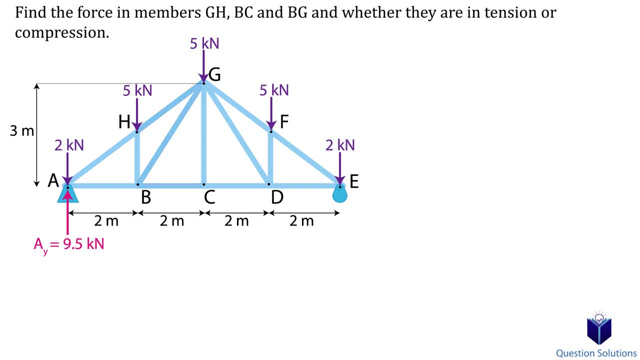 no horizontal forces. Before we do anything else, let's quickly figure out these angles. Notice we can draw a big right angle triangle like this Using the inverse of tan. we can figure out this angle Now. notice that this angle would be the same, since if we create, 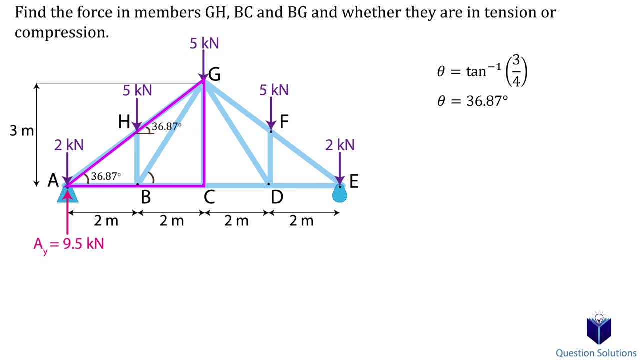 a right angle triangle. like this: it's a similar triangle. The bottom angle can also be found using inverse of tan. Now, these are the forces we need to figure out, so the best place to make a cut is right through them. like this, We can forget about the right side. 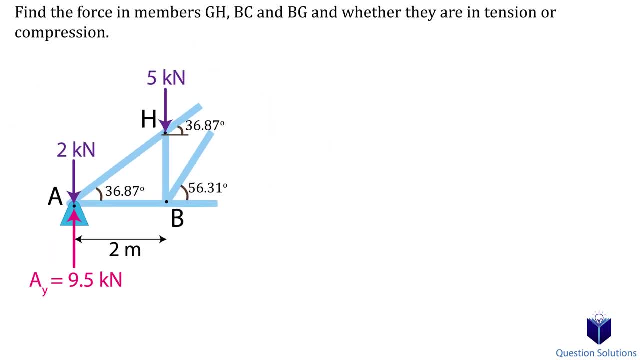 and just focus on the left side. Now I'm going to assume that the forces in our cut members would be like this: Here you have to think of this as being our truss and these cut members as external forces being applied to our truss. So these are internal forces and these are external forces. 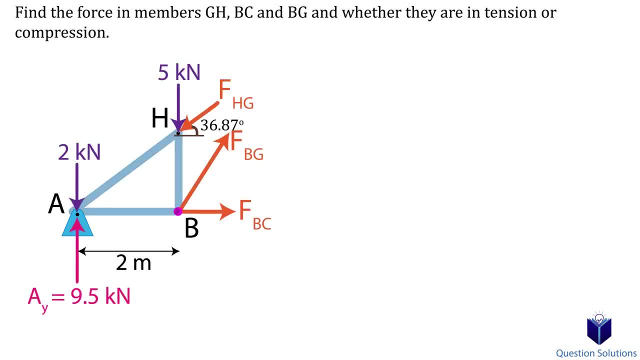 Now let's start with the moment equation about point B. That would eliminate forces BC and BG. It also eliminates the 5kN force being applied, since its line of action goes through point B. Again, note that the force in member AH is an internal force, so we don't need to worry about it. 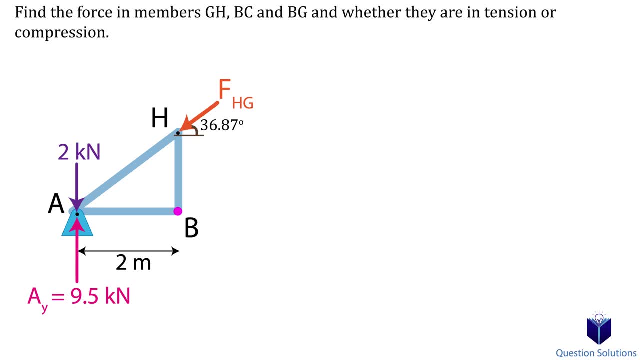 It's the same as when we wrote a moment equation to figure out the reaction at A, We didn't care about the internal forces. in the same way, when we write our moment equation about point B, we don't care about the internal forces in member BH or AH. This leaves just force HG and the reaction at A. 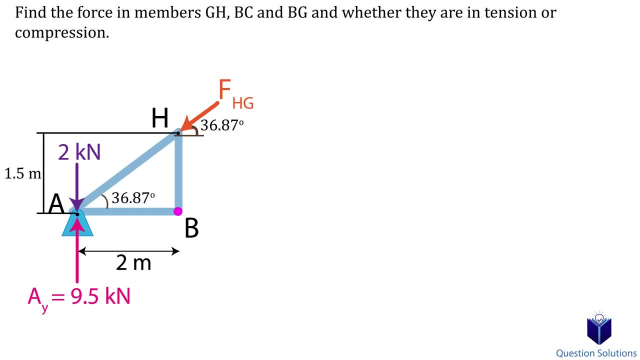 We also need to figure out this height. that can be found by using the angle we found earlier, giving us 1.5 meters. Now let's write our equation and we will pick clockwise to be positive. So we have the vertical reaction at A times the perpendicular distance to pin B, Then we have the 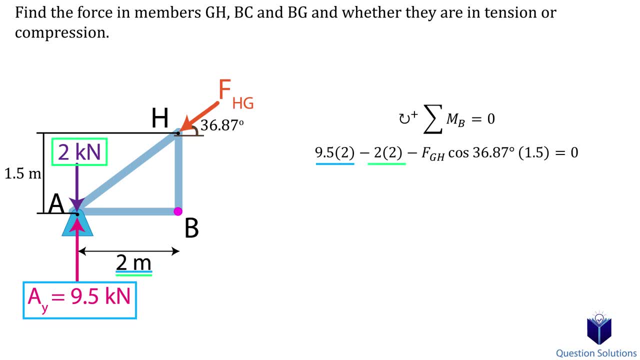 force applied at A times the perpendicular distance. this force creates a counterclockwise moment, so it's negative. Lastly, the force applied yt the angle and the angle we found earlier. we have the x component of force: Hg times the perpendicular distance. The y component does: 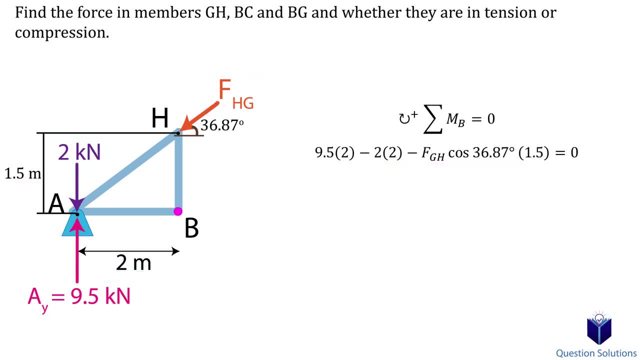 not create a moment, since its line of action goes through point B. Let's solve. We got a positive value, which means our assumption was right and that also means this member is in compression, since the force is coming towards pin H. Remember, when a force comes towards the pin, the member is. 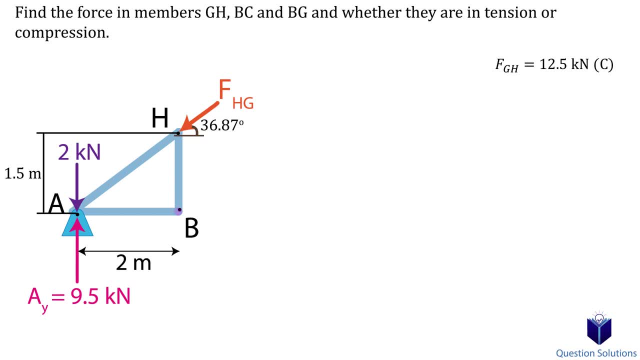 in compression. Now we can write a moment equation about pin A. That would eliminate forces Hg and bc, since their line of action goes through pin A, leaving us with just force Bg. Again. member Bh does not matter to us, since it's an internal member. Note that only the y component. 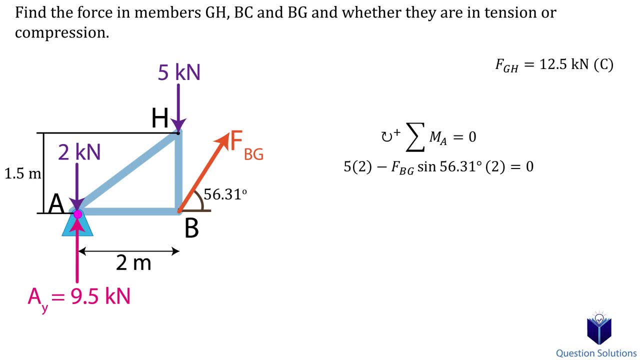 of force Bg creates a moment, since the x component's line of action goes through pin A. Also, the reactions at A are eliminated, since their lines of action goes through pin A. Let's solve: We got a positive value, which means our assumption was right, and since this force is, 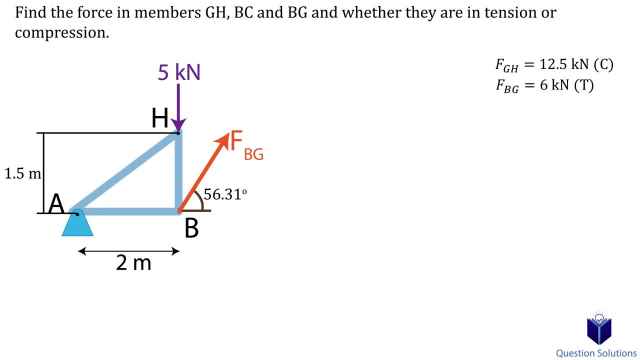 leaving pin B. it'll be intended to create a moment from pin A. Now, if we consider this moment on pin B, the actual force we are creating is the lines of action of Bg and the source of. We figured out two of the three members, so let's find the last one. 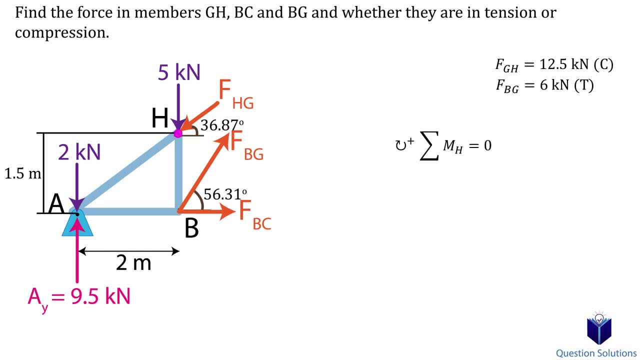 For that we can write a moment equation about point H That eliminates force Hg along with the 5 kN force applied. Note that only the x component of force Bg creates a moment. Let's solve. We got a positive value, so our assumption was right. and since the force is leaving, 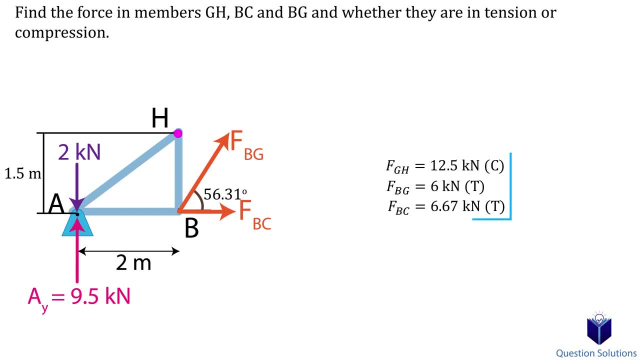 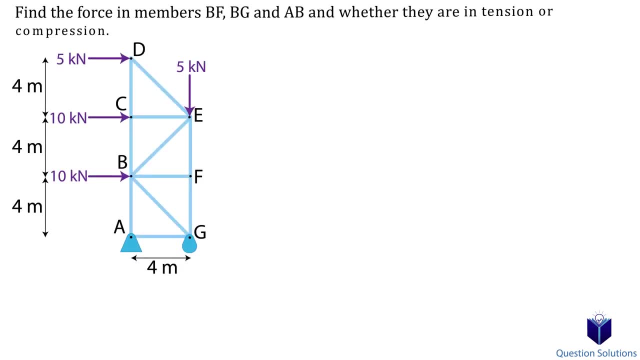 pin B, it'll be in tension. We now solve for the required members using just three moment equations. Let's take a look at this problem, where we need to find the force in members Bf, Bg and Ab and determine whether they're in tension or compression. 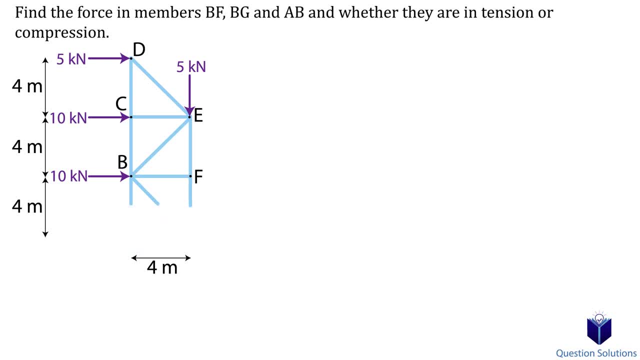 Now I'm going to cut the truss right here and forget about the bottom part. The reason is, if we just focused on the bottom, we'd have to figure out the reactions at the pin and roller. Now I'm going to assume the directions of the forces. 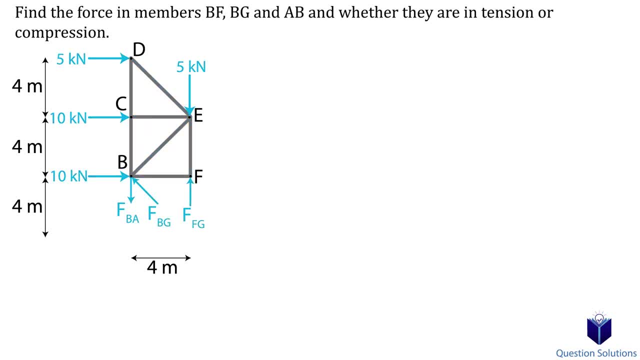 As before, this part is our truss and these are external forces. First let's write a moment equation about point B. Doing so, we'll get a moment equation about point B. The moment equation eliminates the 10kN force being applied at pin B, along with forces. 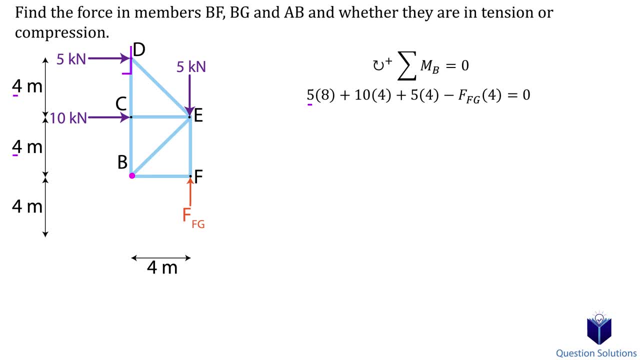 Bg and Ba, leaving us with just force Fg. This will help us figure out the unknowns. we require To figure out the force in member Bg. we need to eliminate force Ba. We can do that by writing a moment equation about point D. 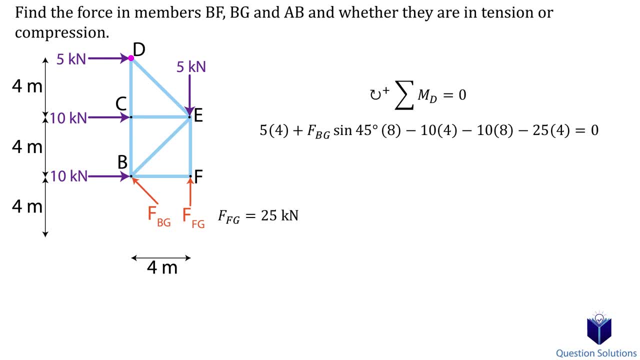 Note that only the x component of force Bg creates a moment about point D. We know the angle is 45 degrees, since it's a moment. The angle is 90 degrees, since its a 90 degree angle divided by 2.. 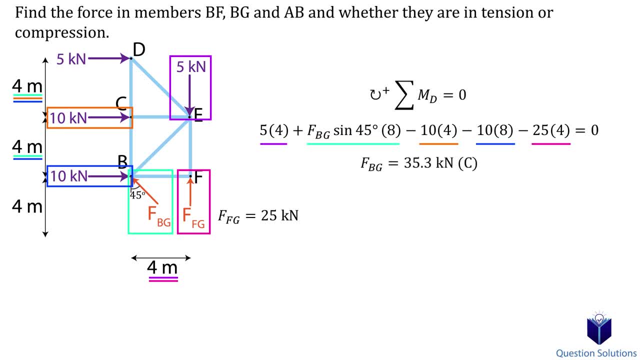 Let's solve. Since we got a positive value, our assumption was right and the force is coming towards pin B, which means the member is in compression. To figure out member Ab, we can write a single equilibrium equation for the y-axis forces. 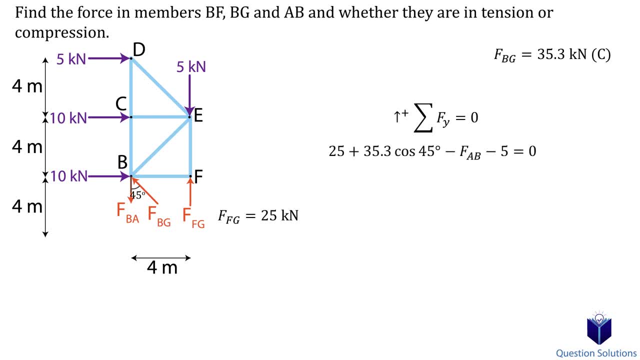 Again, we're considering just external forces. So we have the force Fg, which we already found, and then the y component of force Bg, force BG, which we also found, and lastly the 5kN force applied at point E- Note that we picked. 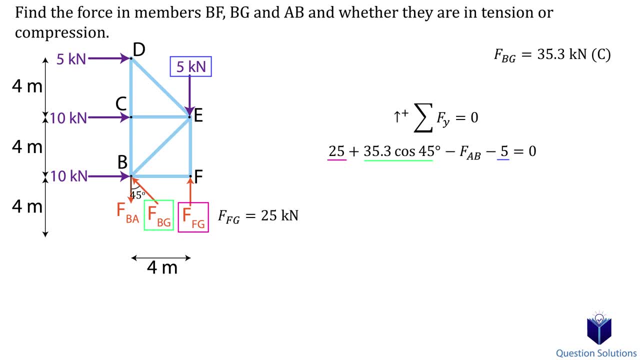 up to be positive, so the 5kN force and force AB are both negative since they point downwards. Let's solve. We got a positive value, so our assumption was right and since it's leaving pin B, the member is in tension. Figuring out member BF is very easy. All we need to do is 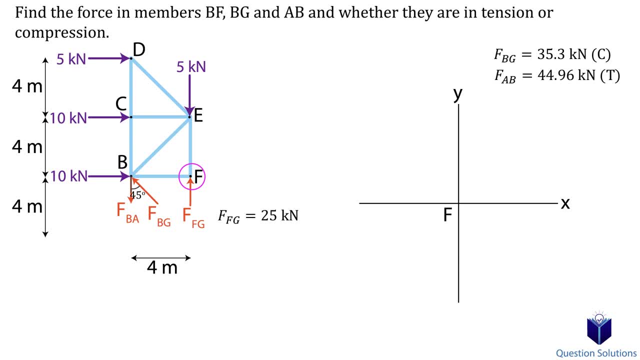 isolate joint F, just like we do in the method of joints. We have force EF, FB and FG. Notice how we have no other horizontal forces. In other words, there is no force being applied in the x-direction. so if you write an equation of equilibrium for the x-axis forces, the only 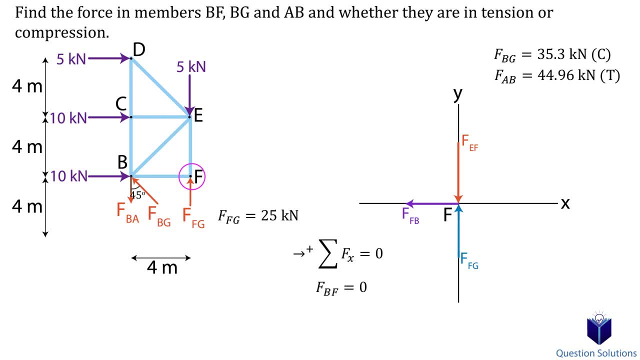 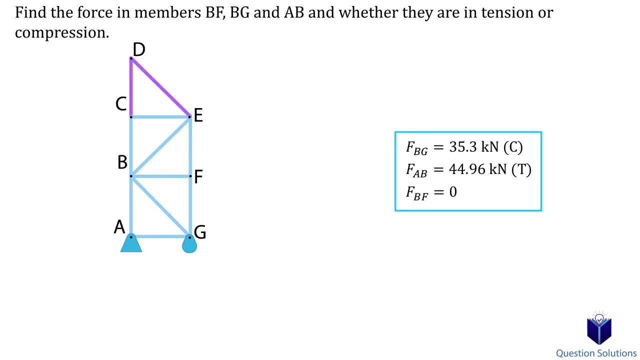 force we have is BF, which means it's zero. So that's a zero force member, And those are our answers. If we were to solve this using the method of joints, we'd have to start up here and solve for all of these members. 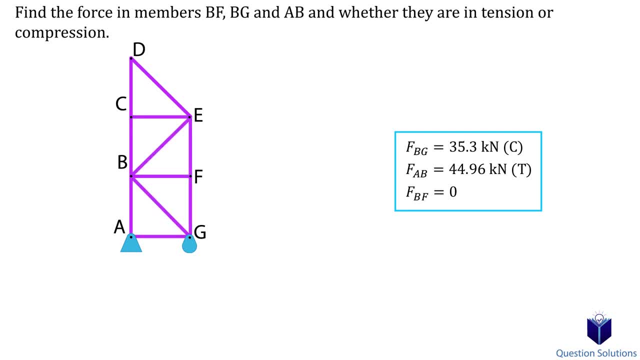 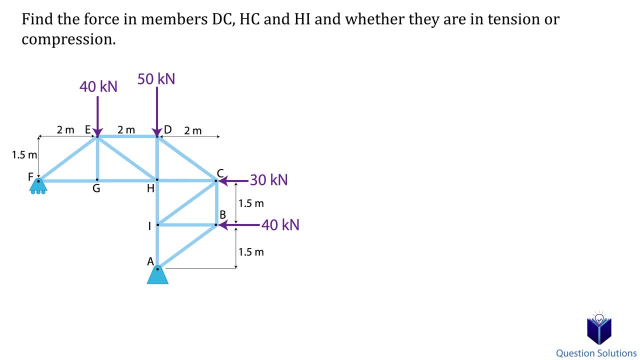 Until we got to the very last ones. Using the method of sections, we solved for the required members using just 4 equations. Let's take a look at this example. In this problem we need to figure out the force in members DC, HC and HI and determine whether the members 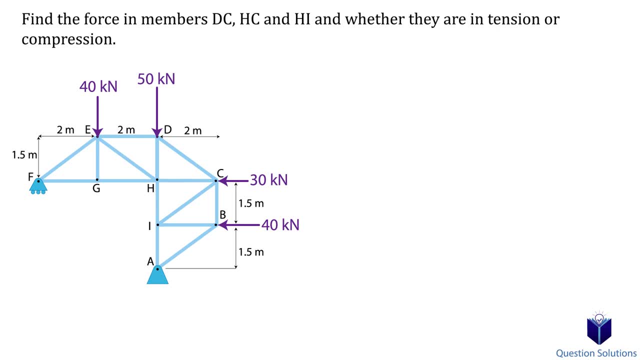 are in tension or compression. First we need to figure out the reactions at the roller. To do that, let's write a moment equation about point A. To begin, we need to figure out this angle. We can use the inverse of tan to do so. Let's solve Now. these are the members. 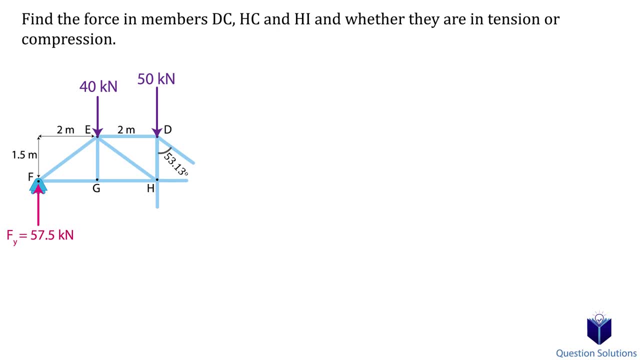 that we need to figure out. so I'm going to cut right here. I'm going to assume these directions for our forces. Now we will write a moment equation about point H. This eliminates forces HC and HI, leaving us with force DC to figure out. Note that the 50kN force is. 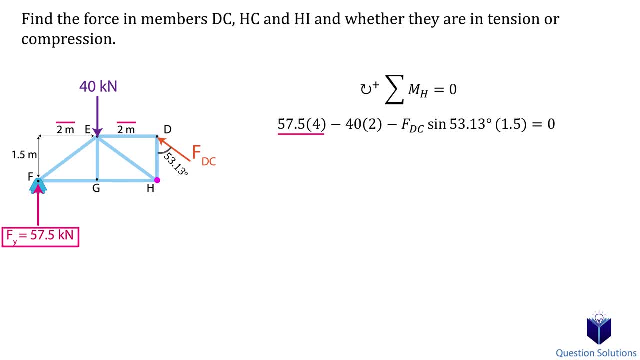 also eliminated, since its line of action goes through pin H. Let's solve, Let's solve. Our assumption was right and since the force is coming towards pin D, that means this member is in compression. Next, we need to find the force in member HI. We can do that by writing an equation. 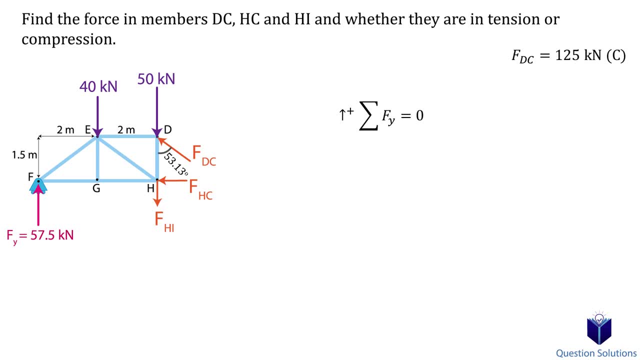 of equilibrium for the y-axis forces. So we have all the external forces, including the y-component of force DC. Let's solve. We got a positive value, so our assumption was right. so that means the member is in tension since the force is leaving pin H. 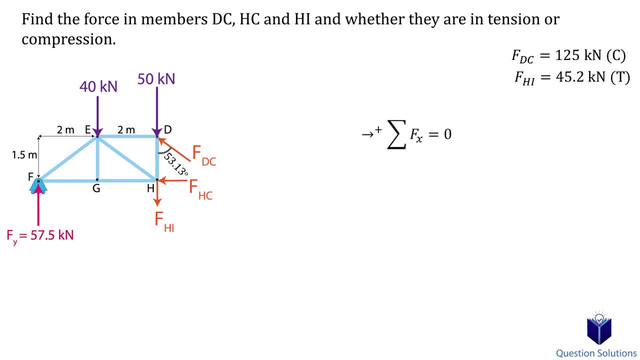 We can do the same to find force DC hc. this time an equation for the x-axis forces. Other than force hc, the only other x-axis force is the x-component of force dc. Let's solve. Notice that we got a negative value.